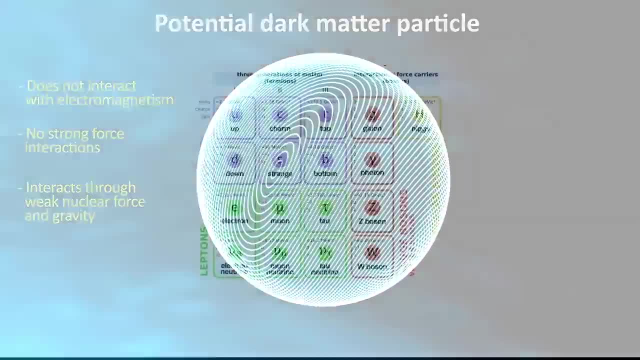 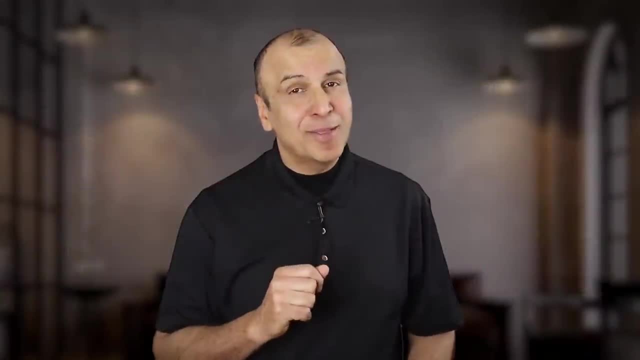 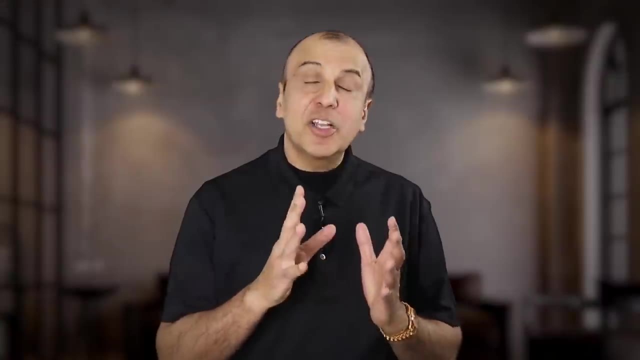 dark matter particle. What is supersymmetry? Why is this idea important And how would it allow us to better understand the nature of the universe That's coming up right now? Let's first understand what symmetry means. in physics, A symmetry exists. if you can. 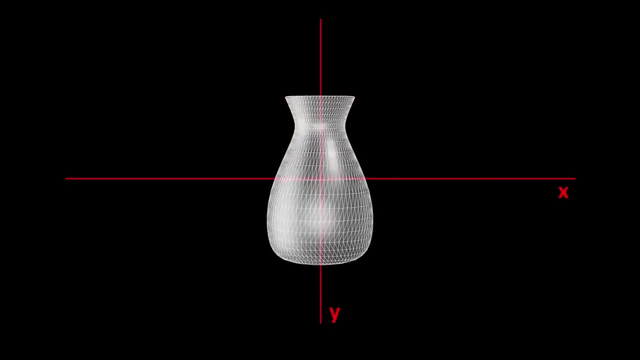 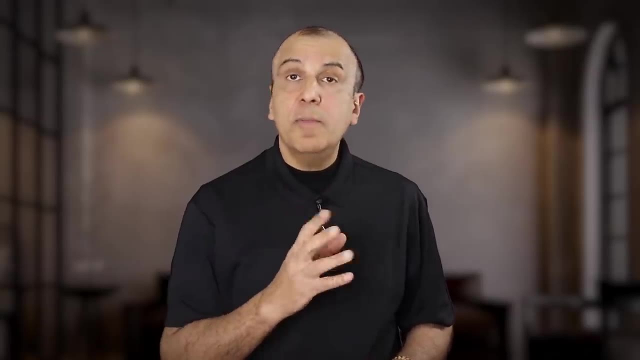 make a change, and that change makes no difference. The physics governing the laws of the universe seem to be based on symmetry. For example, physicists have identified several fundamental symmetries in nature. Three of the more important symmetries are charge. 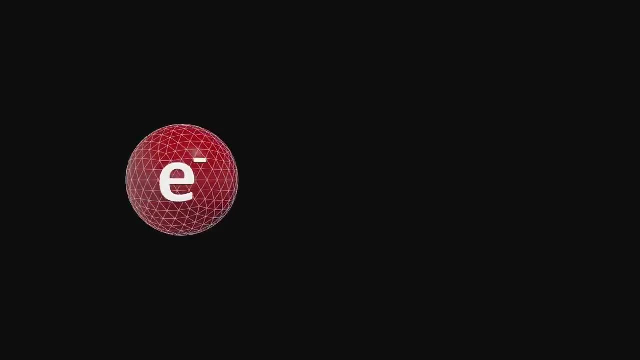 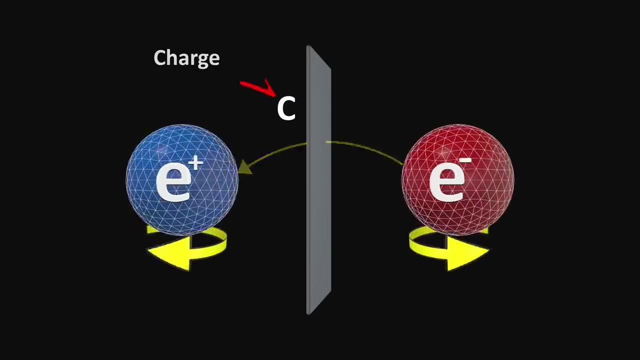 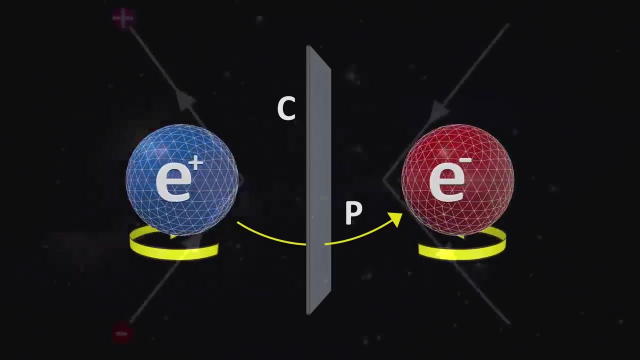 parity and time Charge. symmetry means that if you flip the charges of all the particles involved in an interaction to their opposite charge, you'll get the same interaction. Parity is the idea that if you look at the mirror image of an interaction, you get the same result, And time symmetry is the 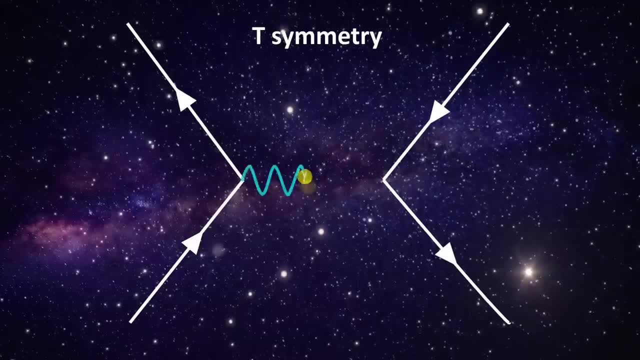 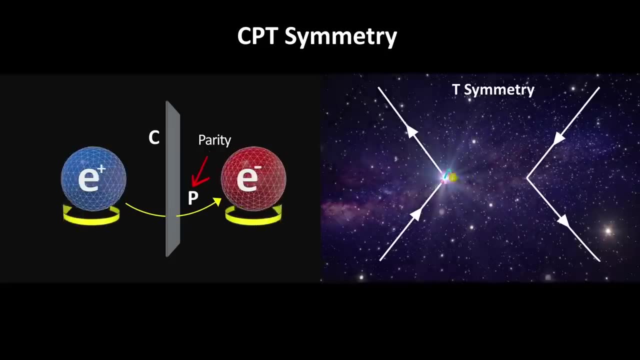 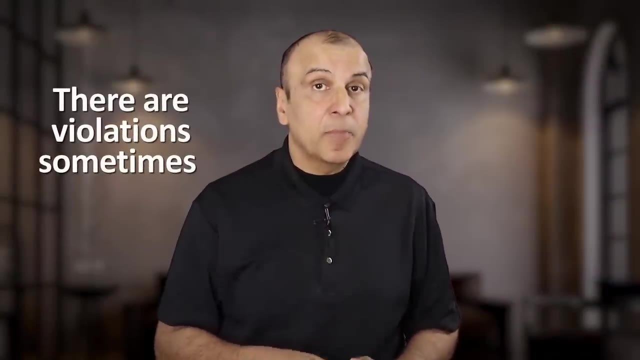 observation that if you run an interaction backwards in time it looks the same Together. they are called CPT for charge, parity and time. Physical interactions obey most of these individual symmetries. most of the time, but not all the time. There are violations sometimes. 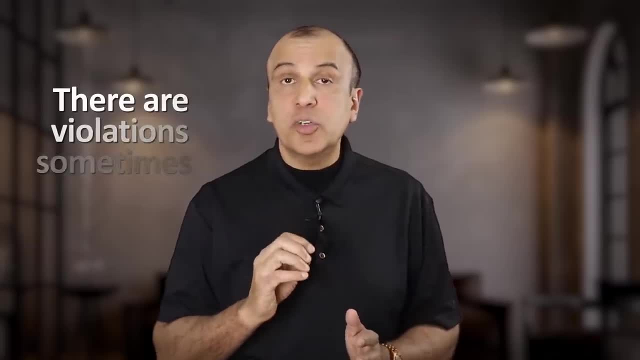 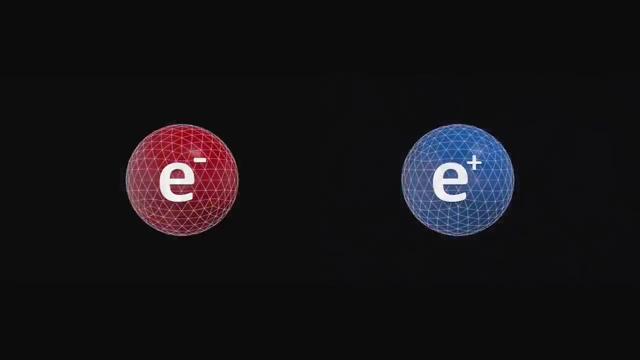 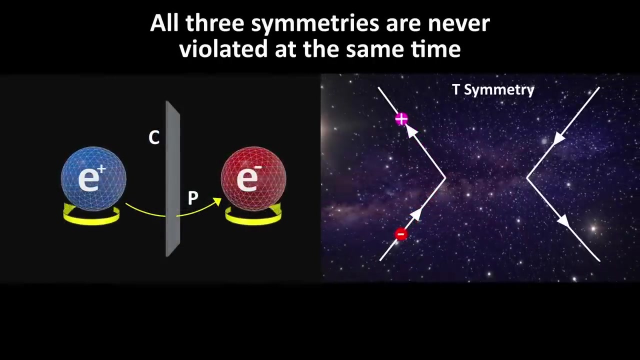 But physicists have never observed a violation of all three symmetries, that is, CPT symmetry, at the same time. This means that if you take every single interaction observed in nature, flip the charges, take the mirror image and run it backwards in time, those interactions behave. 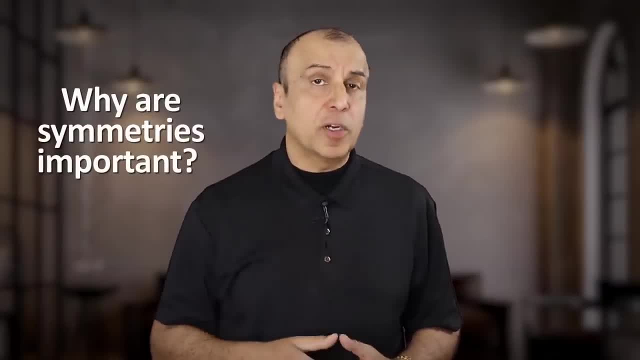 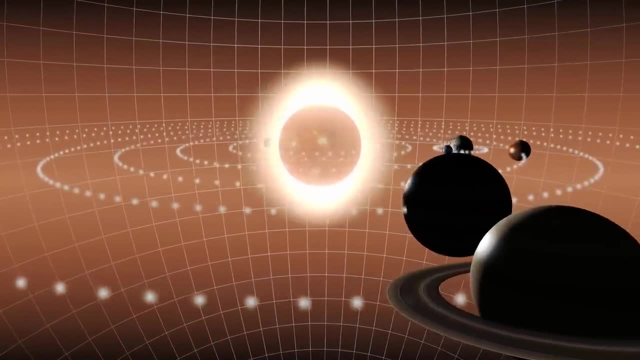 exactly the same. Why are symmetries important in our desire to find a theory of everything? Because if we find that the universe respects certain symmetries, then it will lead to new rules that the universe obeys, And this would limit the number of ways that the universe could. 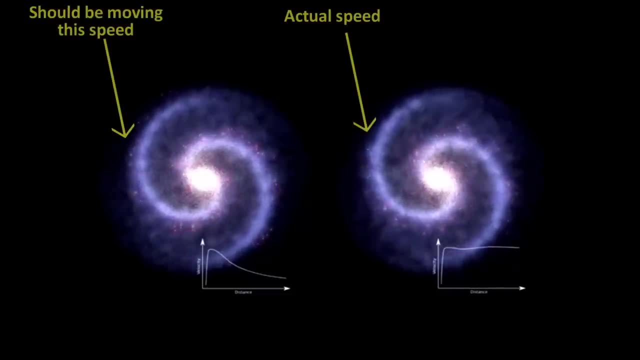 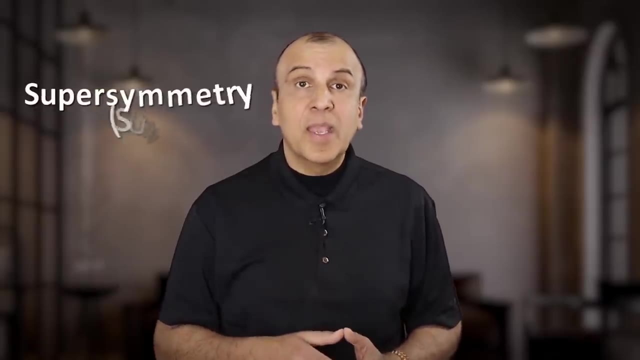 be organized. It would lead to new predictions that would better point us in the direction of the more likely theory of everything. Supersymmetry, or SUSY for short, is a symmetry between matter particles and force particles In the standard model. 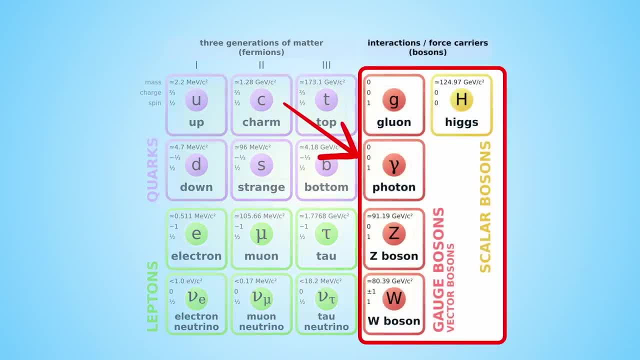 the matter particles are the fermions on the left side and the force carrying particles are the bosons on the right side. The key difference between these two types of particles is spin. All matter particles in the standard model have a spin of a half. 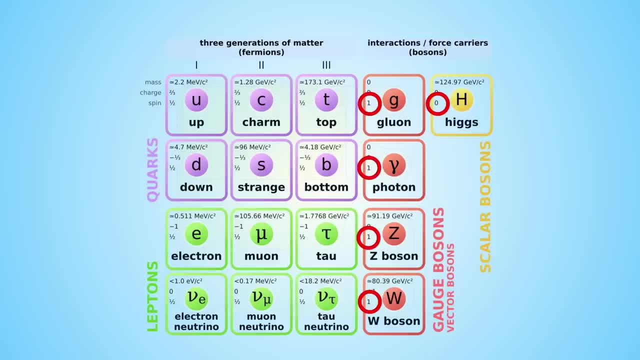 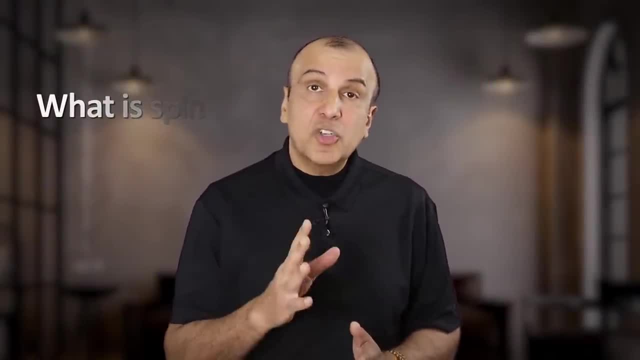 whereas all bosons in the standard model have a spin of zero or one. What is spin? Spin doesn't mean that the quantum object is spinning like a planet. It's a term related to the way particles are deflected through a magnetic field. They act. 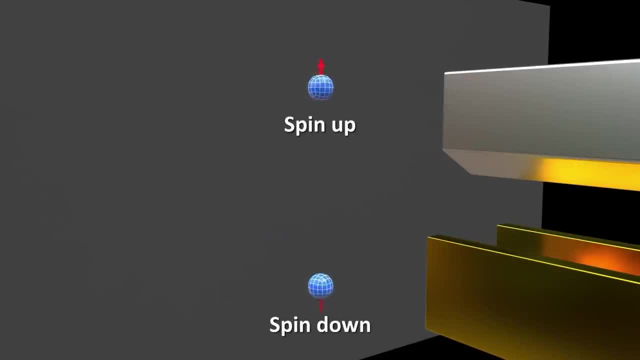 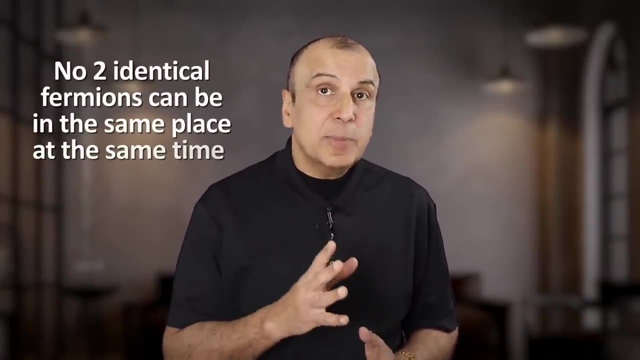 like a spinning magnet, but that is not what's actually physically happening at the quantum level. The rules fermions obey is that no two of them can be completely identical. They can't be in the same spot at the same time with the same spin. This is what the Pauli exclusion principle 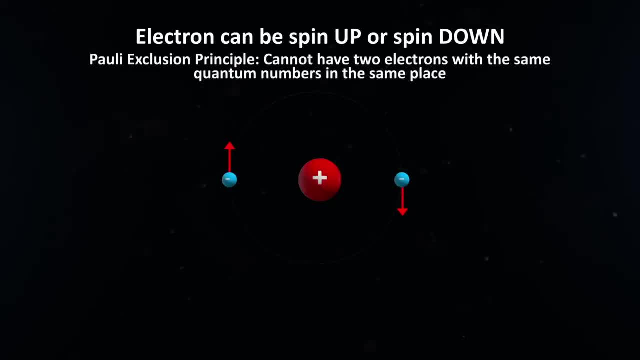 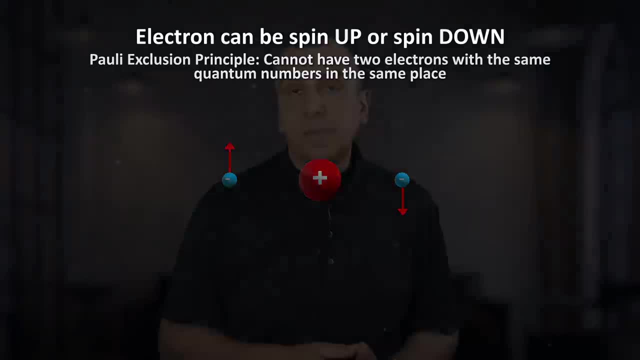 is all about, And this is the reason that only two electrons with opposite spins can ever be in the same orbital in atoms, but never more than two, because then at least two of them would be identical. This rule does not apply to bosons, as many identical bosons can be at the same place? 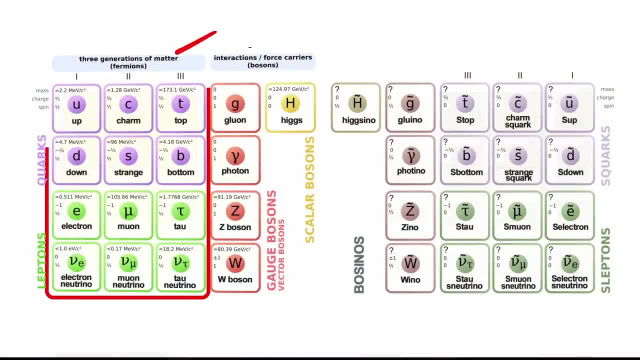 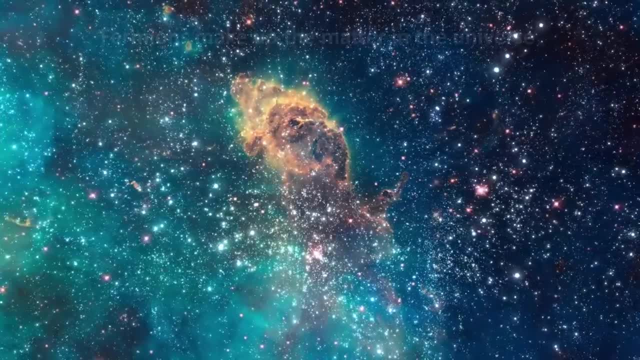 at the same time, The supersymmetric partners of the fermions would be bosons, and so they could be found with others in the same place and time. Fermions are what make up the matter in the universe. Bosons are what carry the forces. 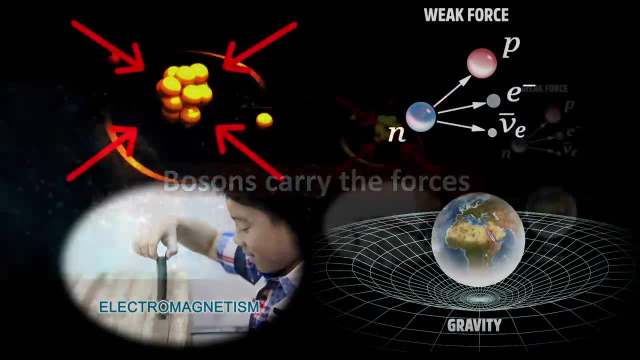 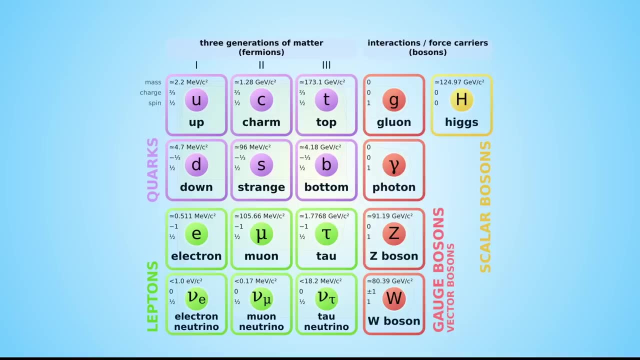 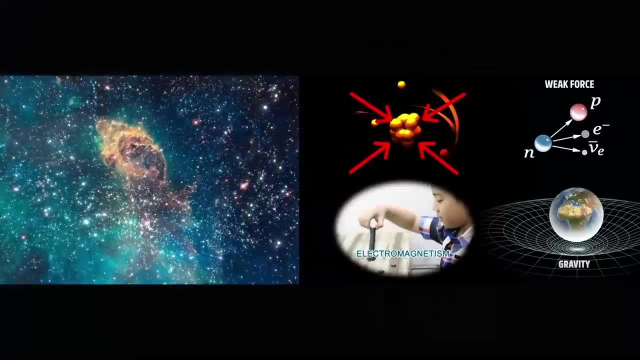 between matter particles. These two classes of particles are quite different, so why does anyone think that they could be treated identically? If you look at the standard model, it seems a bit arbitrary that there should be many more matter particles than force carrying particles. Does the universe favor matter? 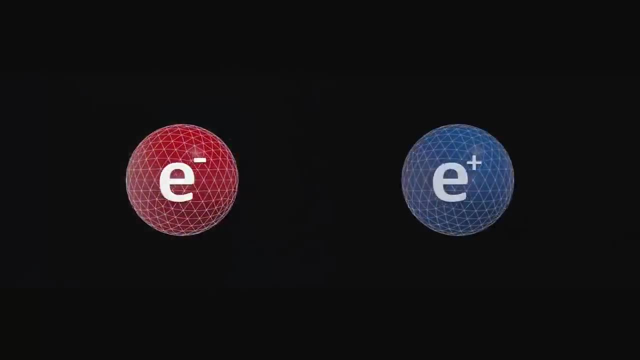 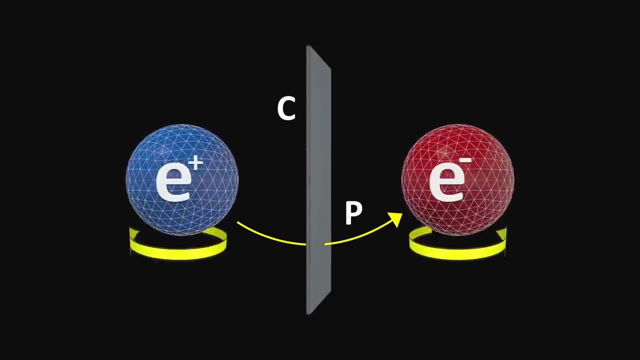 over the forces that allow interactions. Since the standard model is littered with symmetries like time, parity, charge and others, to many physicists it seems that a fundamental symmetry between fermions and bosons should also exist. Supersymmetry is the term used. 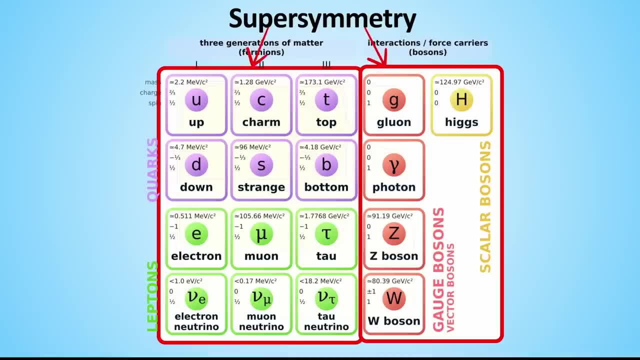 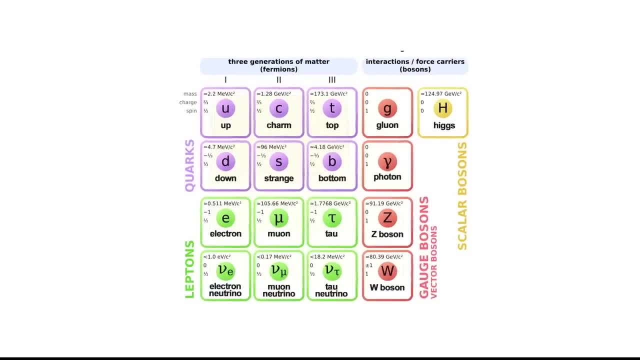 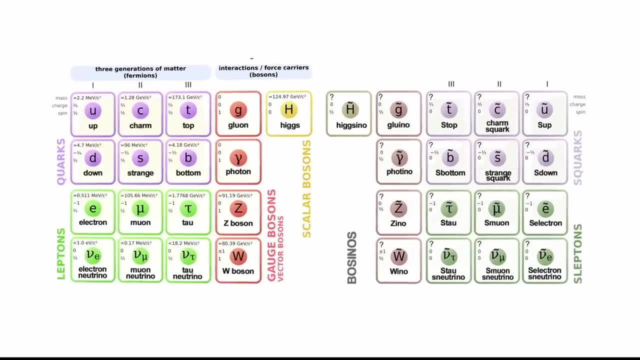 to describe the symmetry between matter and the governing forces. Now there are different flavors and modifications of supersymmetry theories, but the essential concept is fairly simple. We take the mirror image of the standard model. by this I mean that every particle has a mirror particle. 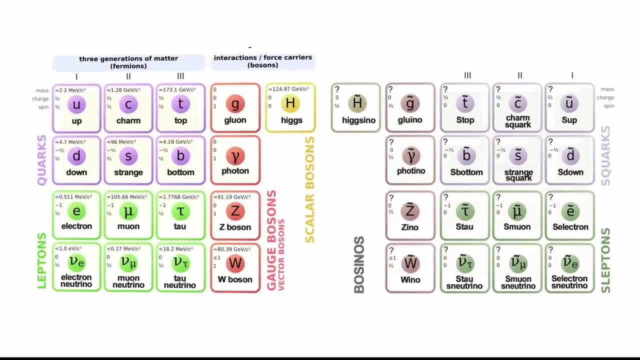 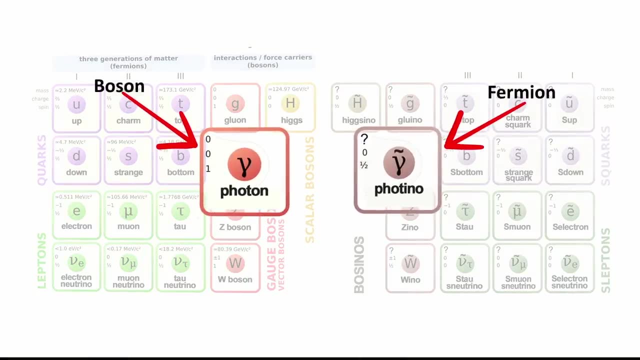 Each mirror particle is of the opposite type. so each fermion has a supersymmetric counterpart, that is a boson. Likewise, all mirror particles of the bosons would be fermions. And with this simple idea of supersymmetry we can bring a balance to the model such that 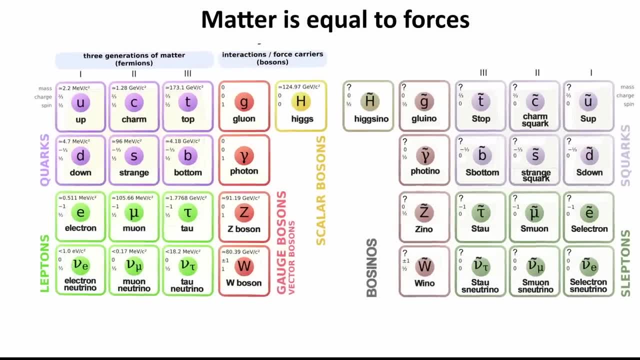 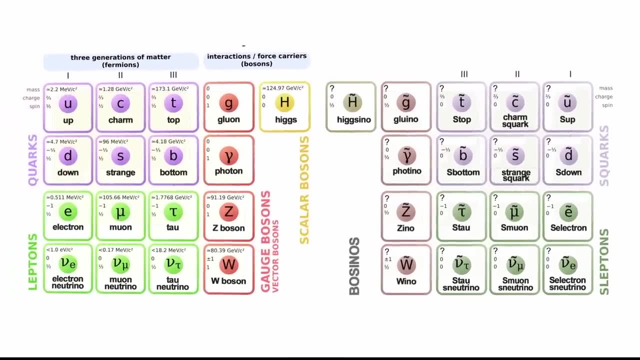 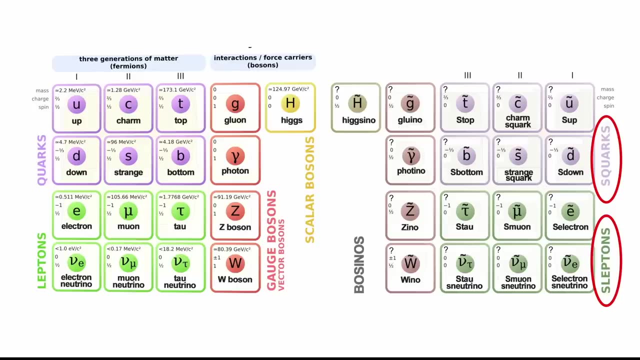 we have the same number of fermions as bosons. Matter is equal to the forces. The naming convention for the supersymmetric counterparts of the fermions is that we end with an S in front of the names of quarks and leptons. So the mirror particles of the fermions which are now bosons are called squarks and sleptons. 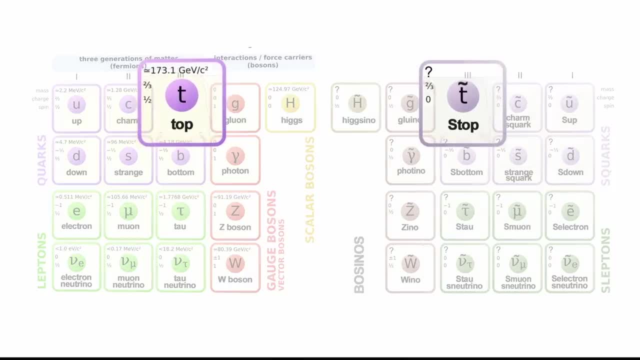 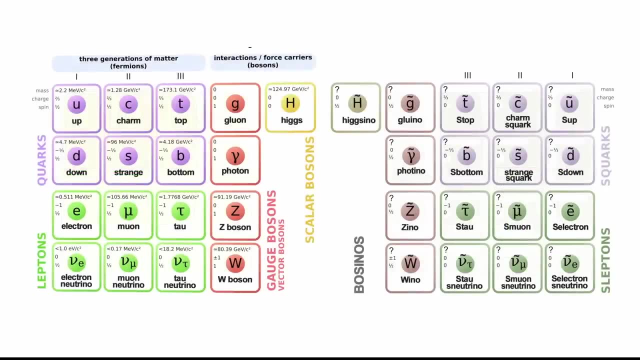 For example, the mirror particle of the top quark is called the stop-squark boson. The mirror particle of the electron is called the selectron boson. Likewise, the mirror particles of the bosons which are fermions get a suffix "-ino" For. 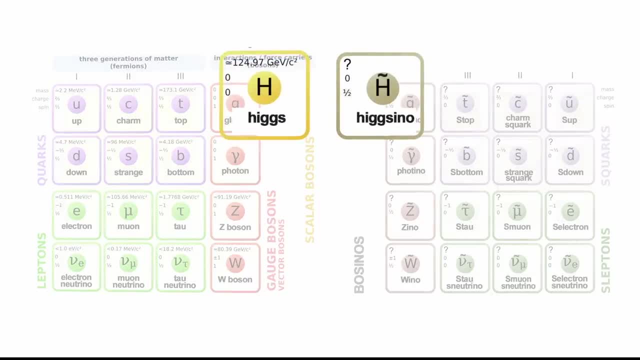 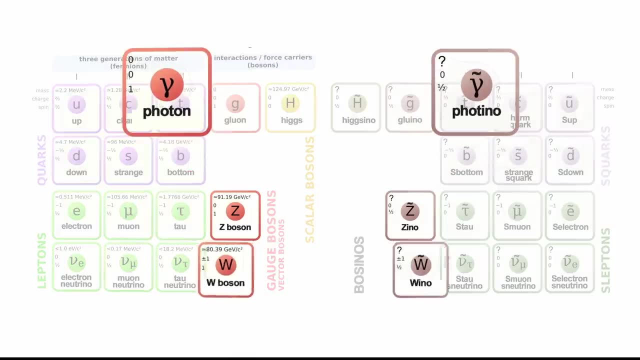 example, the Higgs boson mirror particle is the Hig-xeno fermion fermion and the gluon counterpart is the gluino fermion. Similarly, fortino, vino and zeno. You might ask what is the point of all this? Is it really important that there? 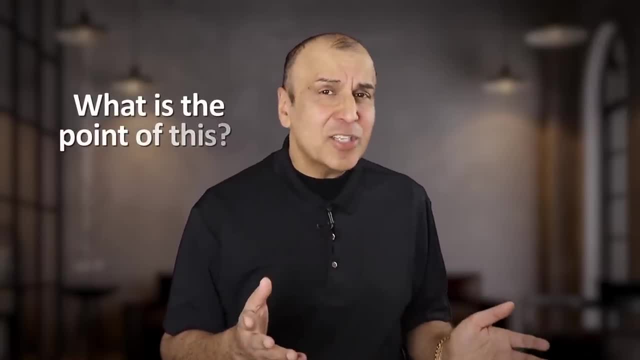 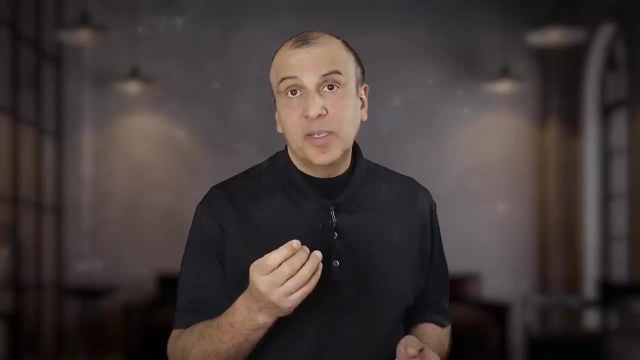 is an equal number of bosons and fermions. Do we really need such a symmetry? Well, we can't be sure of that, but there are some reasons why such a theory could be desirable. It would help us understand the universe better, if it's correct, In the early days of the 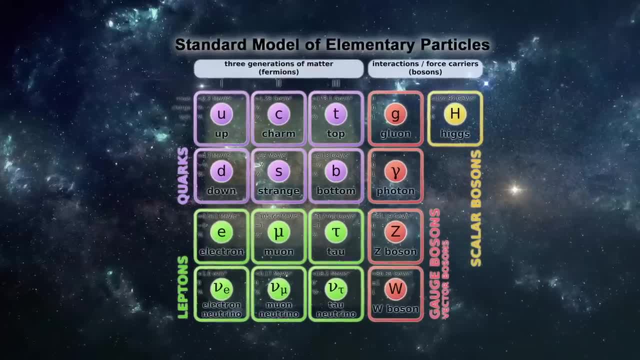 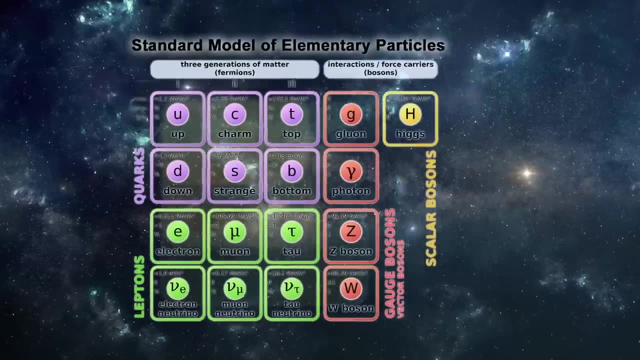 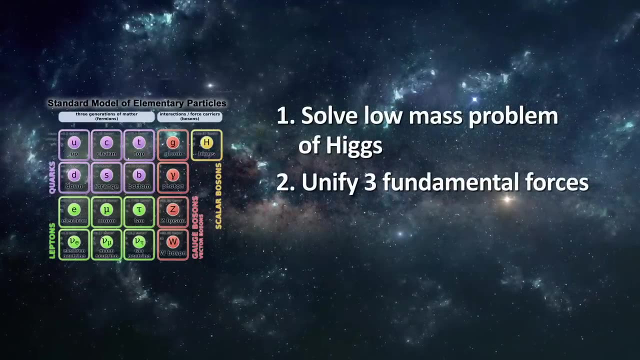 standard model going back to the 80s, physicists had already began to notice some issues with the standard model In general. there are three main reasons why supersymmetry is a good idea. One, it would solve the low mass problem of the Higgs boson. Two, it would unify three elemental forces. 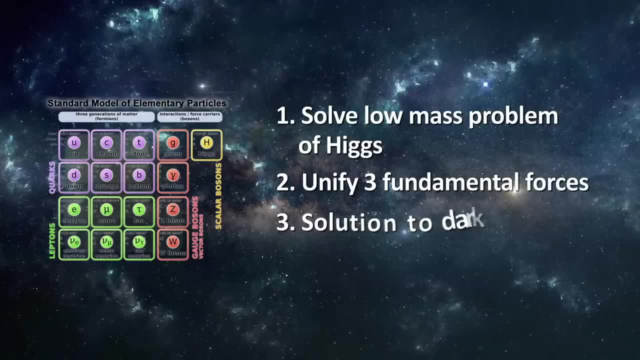 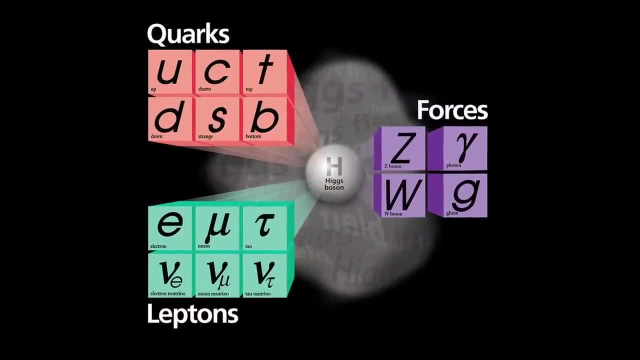 Electromagnetism, the strong and the weak forces. Three: it provides a solution to dark matter. The first problem, in simple terms, is that the mass of the Higgs boson appears unnatural, or at least didn't change when it comes down to it. If you use these solutions, however, 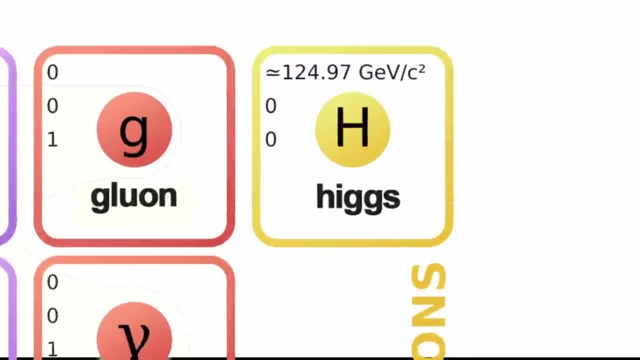 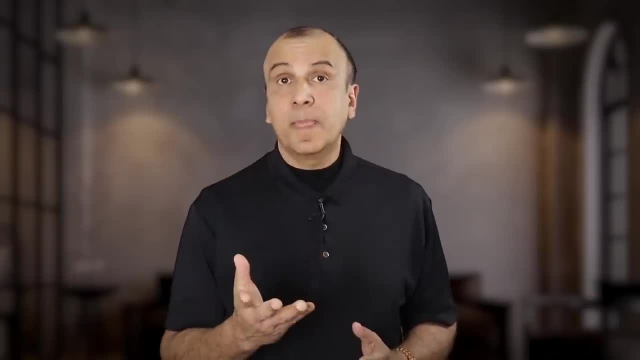 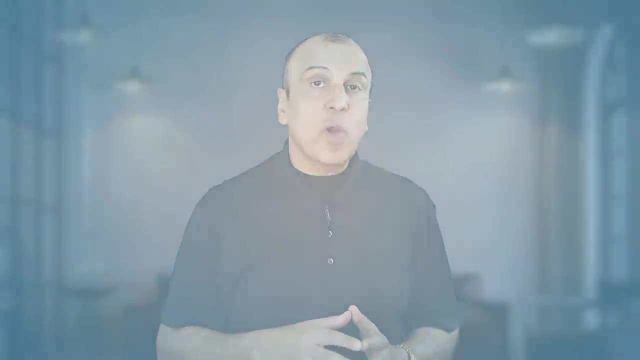 very finely tuned. The Higgs has a mass of 125 gigaelectron volts, or GEV. Theoretically, this seems improbable. Why This is related to how quantum corrections affect the mass of the Higgs boson. In a simplified way, we can write: 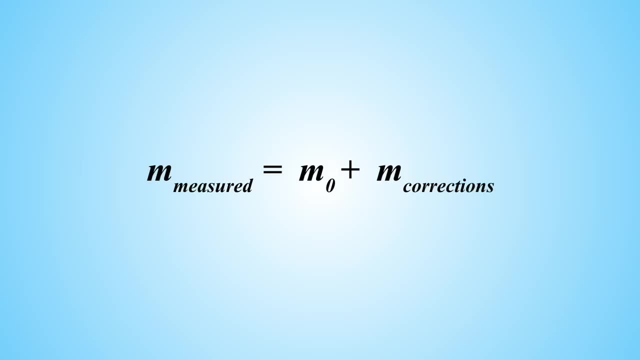 the mass of the Higgs boson as follows: There's a measured mass, which is what we can measure in experiments like at the LHC. M-corrections is the corrections to the mass calculated based on the equations of the standard model, And M-naught is a. 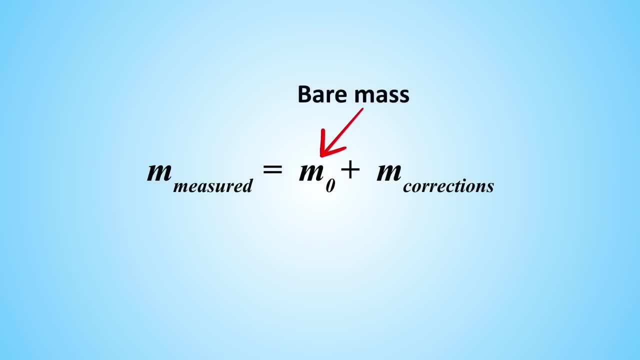 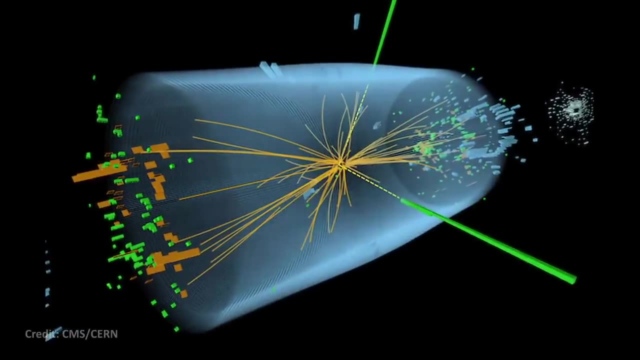 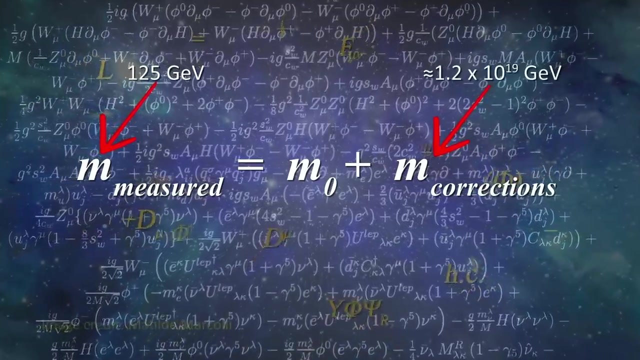 tuned parameter called the bare mass. The standard model doesn't tell us what this bare mass should be. We know the measured mass from experiments at the LHC. The problem is that when we calculate the M-corrections using the equations of the standard model, this turns out to be a very large number, many orders of. 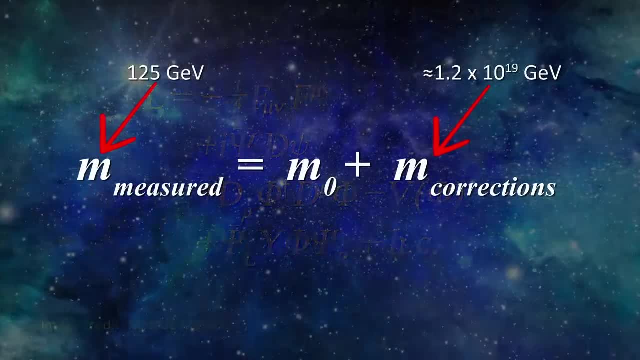 magnitude higher than the measured mass. In fact, based on this, M-naught would not be a very large number. In fact, based on this, M-naught would not be a very large number. In fact, based on this, M-naught would not. 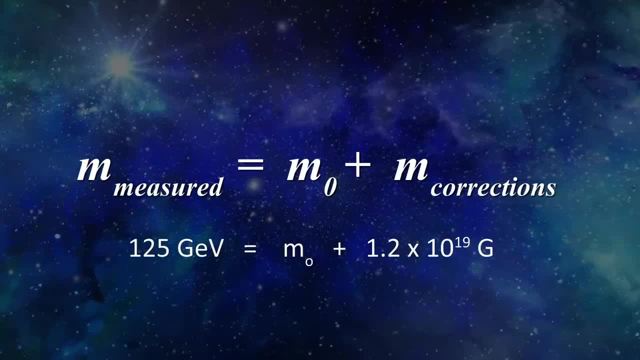 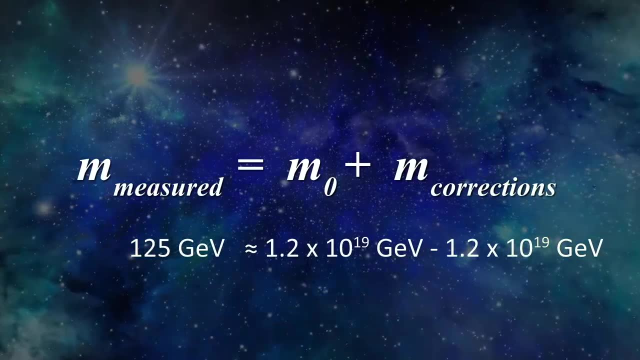 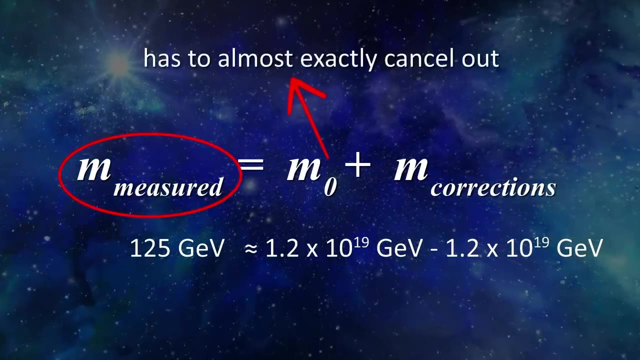 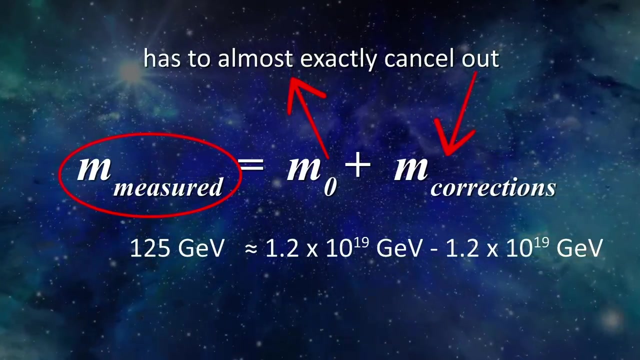 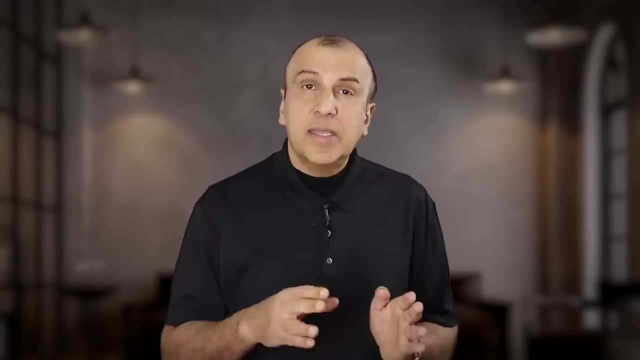 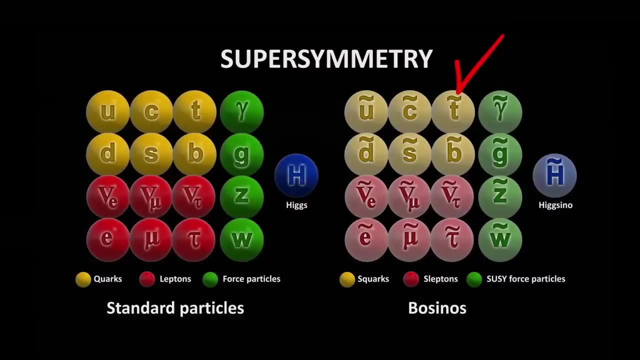 fine tuning or at least an unlikely coincidence. This is where supersymmetry can help better explain the measured mass of the Higgs. Extra bosons from supersymmetry, like the Stop-Squark or some other supersymmetric bosons, could cancel these extremely large quantum corrections. 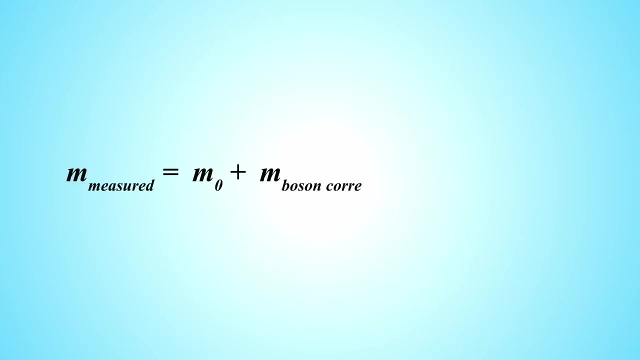 Because bosons contribute opposite the Higgs mass compared to the fermions. This equation highlights this fact. In this case, extra particles from supersymmetry can solve the hierarchy problem because there would no longer be these enormous quantum corrections. In the absence of these quantum corrections, it would make sense that the Higgs is a very 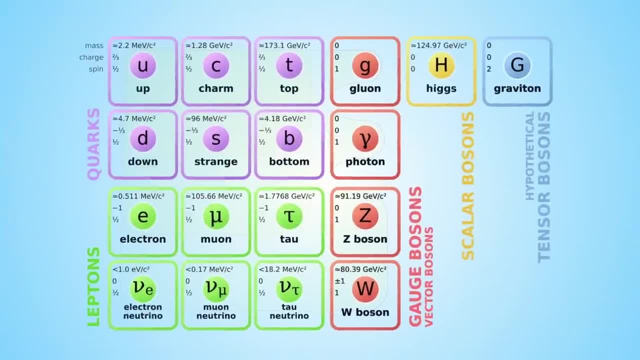 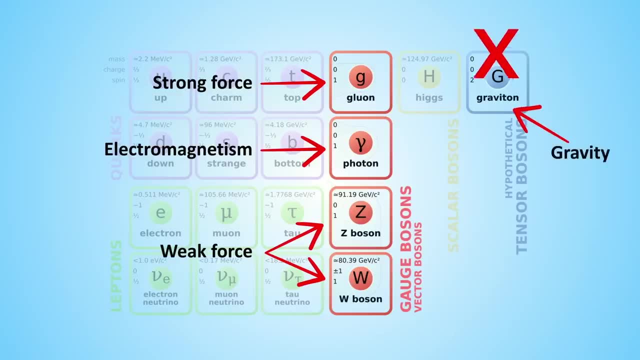 light particle, just like we measured it. Next, there's a question of the unification of forces. The Standard Model accounts for the electromagnetic strong and weak force, but not gravity, And that is another issue with the Standard Model. Physicists believe that at some fundamental level, all forces 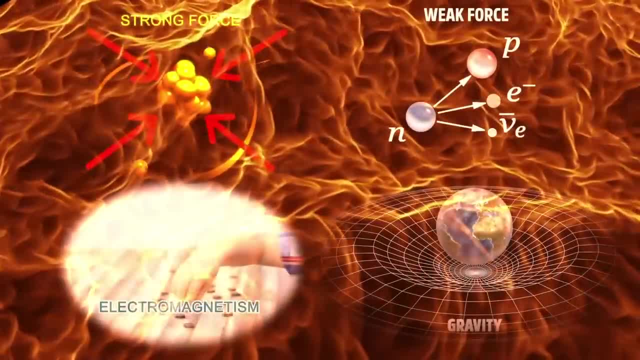 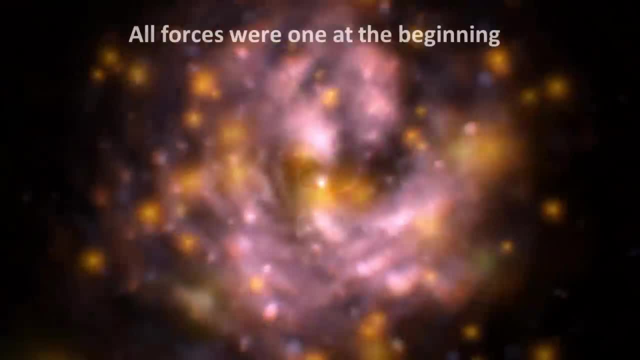 are united and that there is some theory that unifies the forces and explains physics in a unique way. And, as we will be learning from the beginning of this video, many people unified way. We've found good reason to believe that this could be possible, because history has. 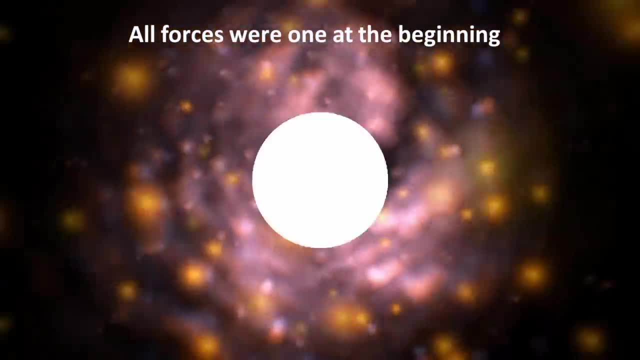 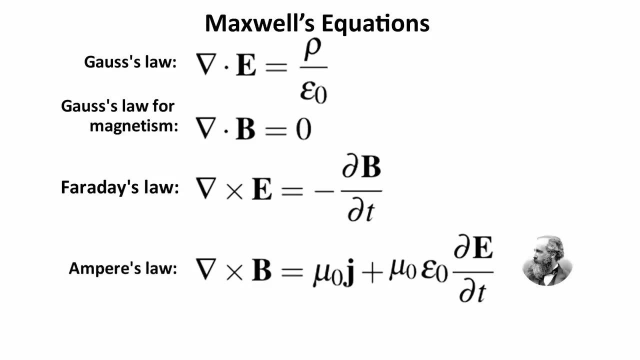 shown us that forces seem to unite at some higher level. For example, James Clark Maxwell unified electricity and magnetism, which were once thought to be two completely different forces, with his equations of electromagnetism. We've since gone further, because in the 20th century, physicists 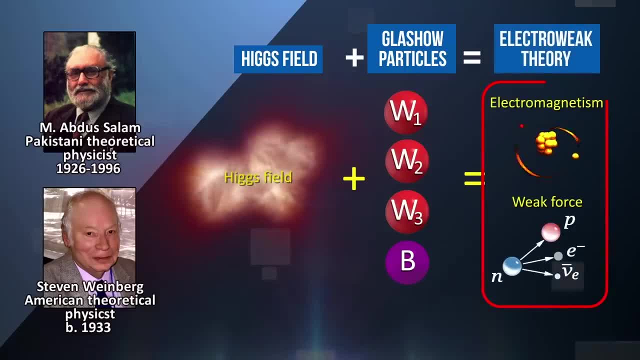 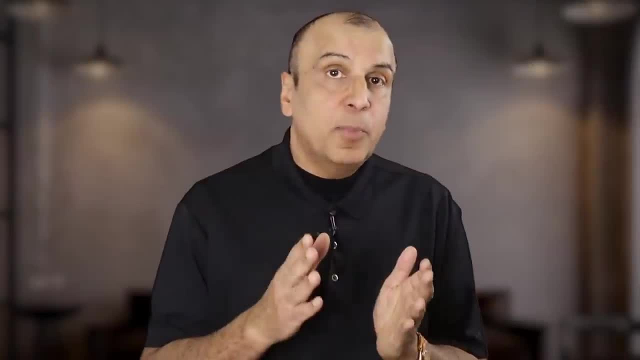 showed with the electroweak theory that electromagnetism and the weak force are also united at a deeper level. So it makes sense that the other forces might also be related in some deeper way, forming a more fundamental unified theory of forces, leading to a theory of. 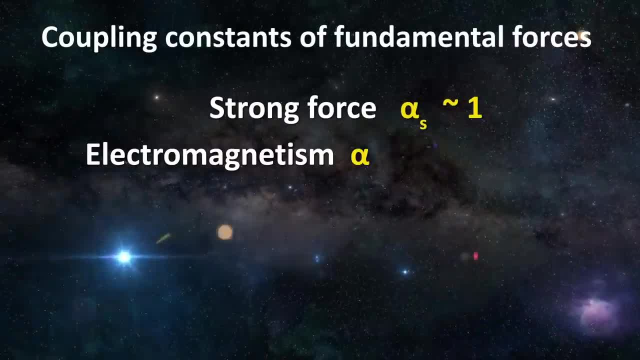 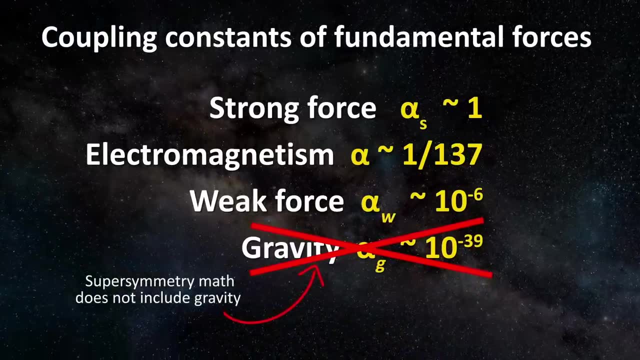 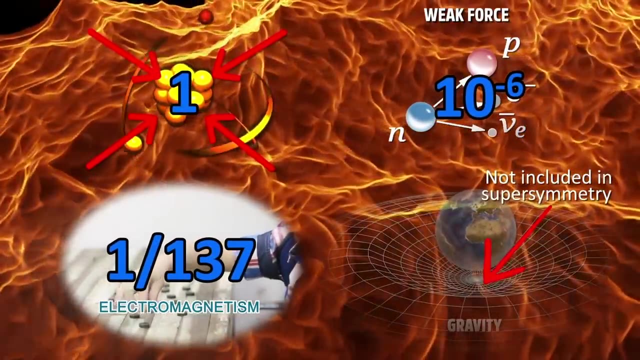 everything. Each force of the standard model has some coupling constant that reflects the strength of the force. These coupling constants are not actually constant because they change at higher temperatures. Physicists expect that the coupling constants should unite at some very high temperature where the forces unite. Thus, at some point, the different coupling constants of the different 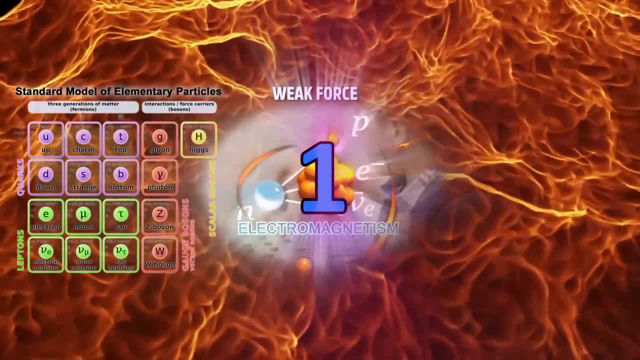 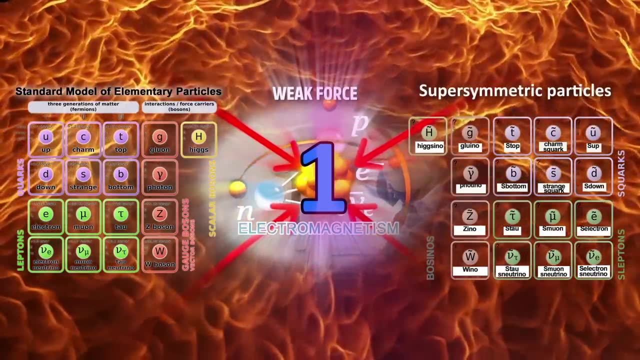 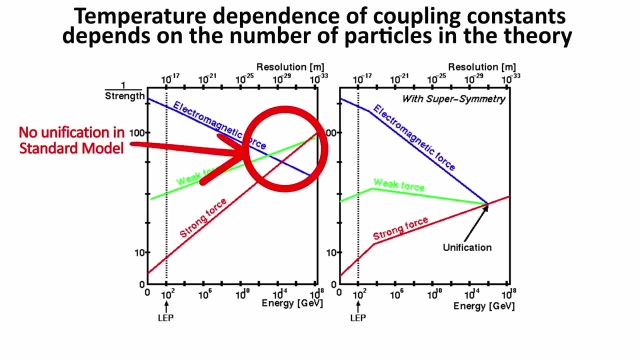 forces should become equal. In the standard model this doesn't initially seem to be the case, but adding the extra particles from supersymmetry could change how the couplings change at higher temperatures such that they might unify at some point. This is because the temperature dependence of the coupling depends. 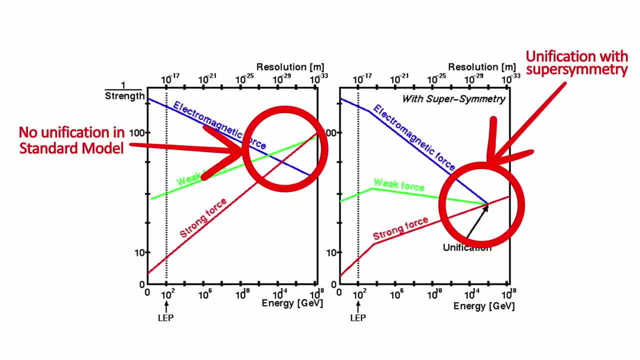 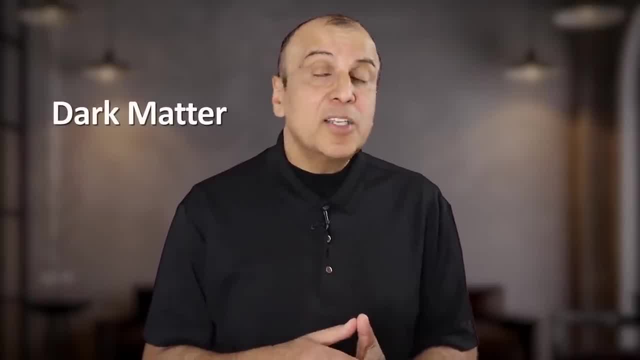 on the number of particles in the theory, and supersymmetry would at least double the number of particles in the theory. Now, finally, there's the issue of dark matter, a problem that has haunted physicists for all of their lives. The problem of dark matter is one that has haunted physicists for 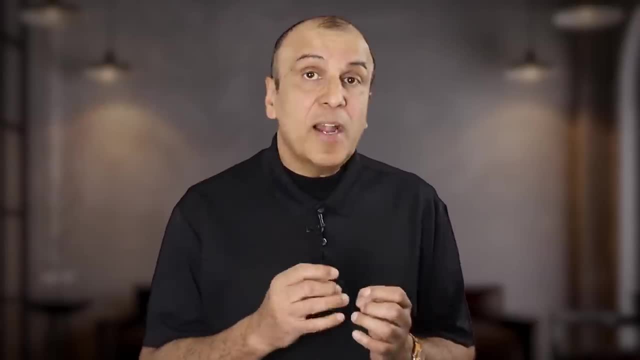 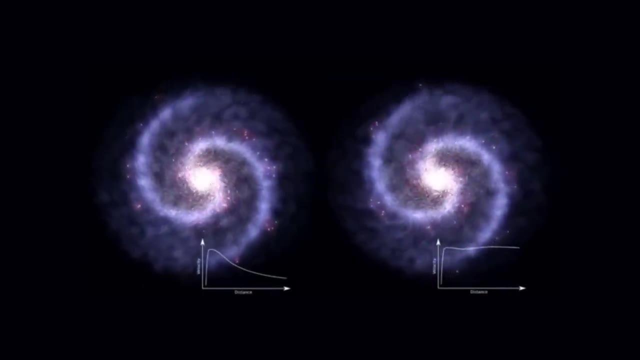 almost a century and we still haven't resolved it. Dark matter, if found, could explain fundamental astronomical observations, such as why our galaxy stays together, even though the stars in the outer edges are moving much too fast. according to Newton's laws, They should fly apart. 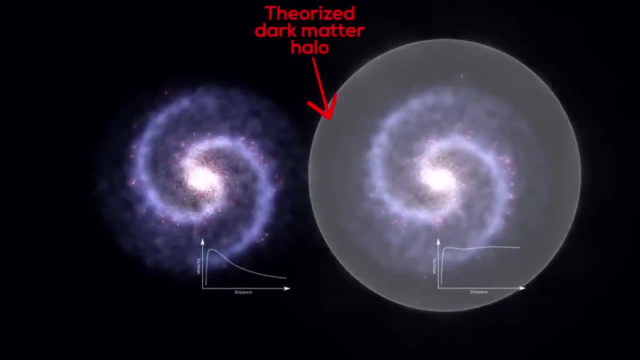 unless there is more matter than we can see. This is called dark matter because we can't see it, And if it exists, it would form a halo around most galaxies. Calculations show that there is at least five times as much dark matter as there is at the surface of the galaxy. It is only 5 times as much. 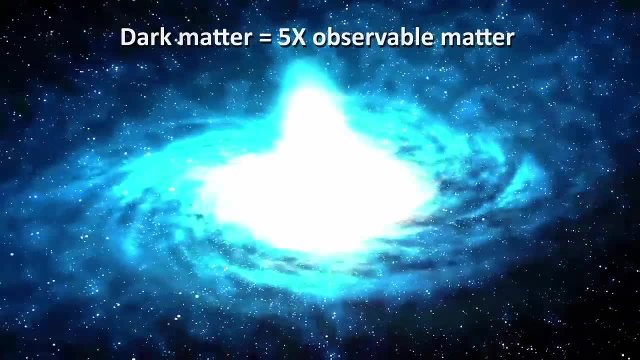 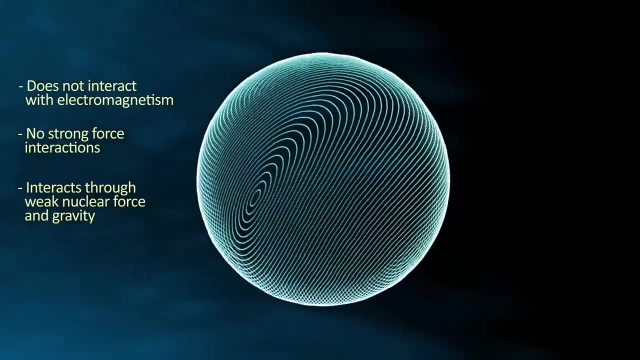 times as much dark matter as ordinary matter. An undetected supersymmetric particle could provide a perfect candidate for this dark matter particle. It has to be stable, electrically neutral and massive. The lightest supersymmetric particle would be stable and very massive. 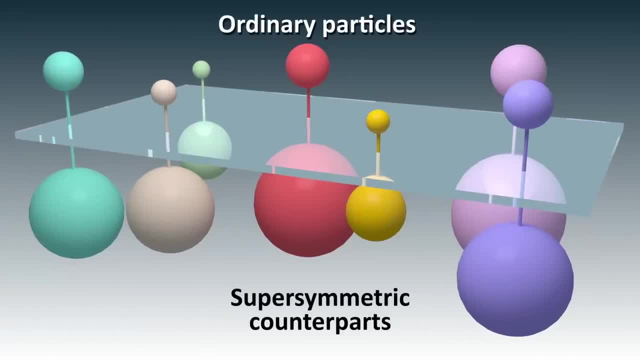 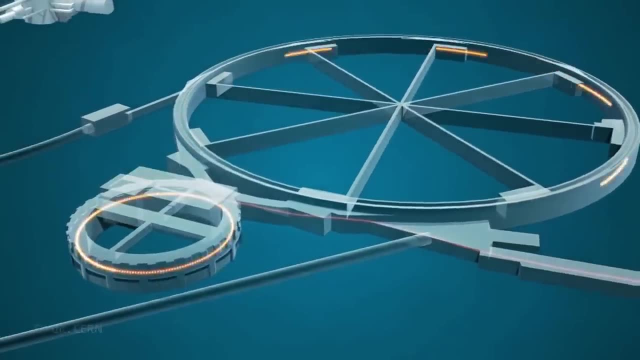 We don't know which particle because we don't know which one is the lightest. Why would supersymmetric particles be massive? Because if they were light particles, we would have detected them in our particle accelerators by now, given the energies that we can produce. 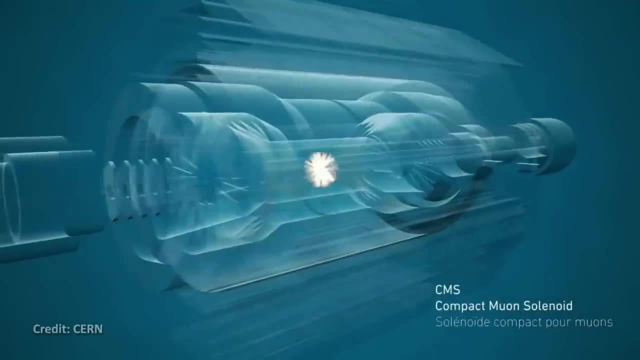 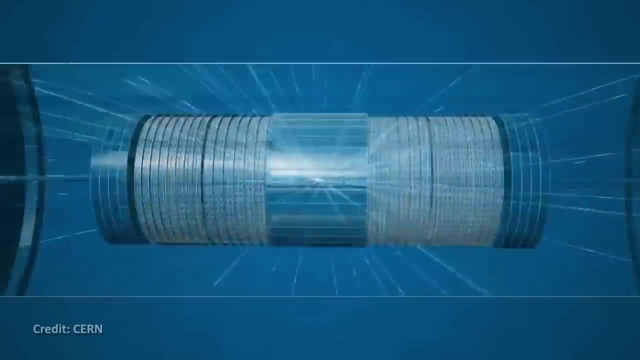 Since we haven't detected them. scientists believe that they must have more energy or more mass than can be produced at our most advanced particle accelerator like the LHC, perhaps a thousand times or more than the mass of the proton. So if the dark matter 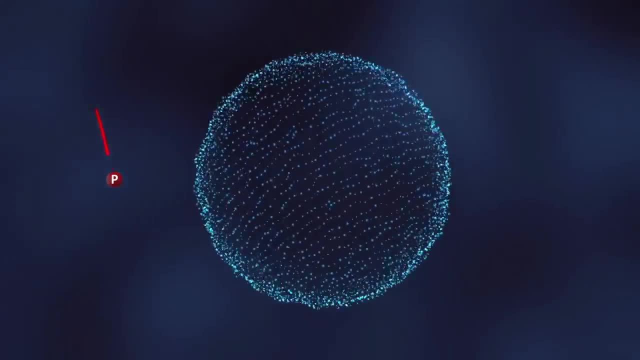 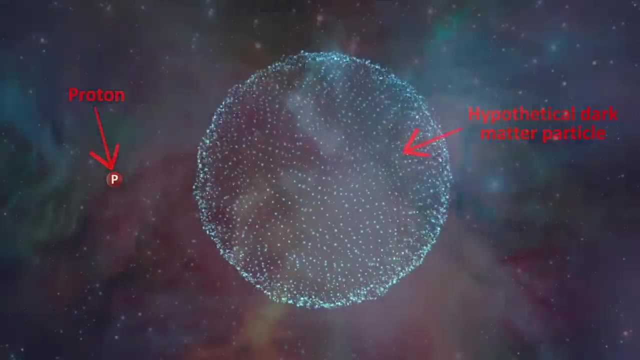 particles are very heavy, then you don't necessarily need that many particles relative to the number of standard particles to have five times more dark matter mass in the universe. This would support the idea that a relatively small number of supersymmetric particles could make a difference. 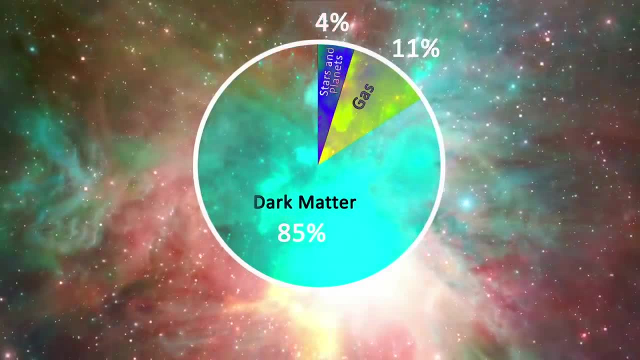 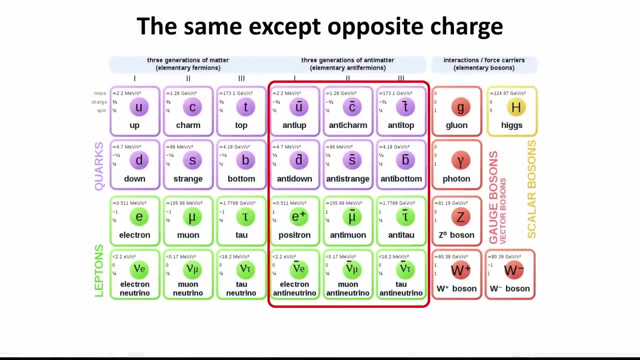 Now let's take a look at the dark matter. density of the universe, You might say. I thought symmetry meant that you change one property but everything else stays the same. like antimatter is exactly the same as matter, but with an opposite charge. So shouldn't supersymmetric particles be just like ordinary particles? 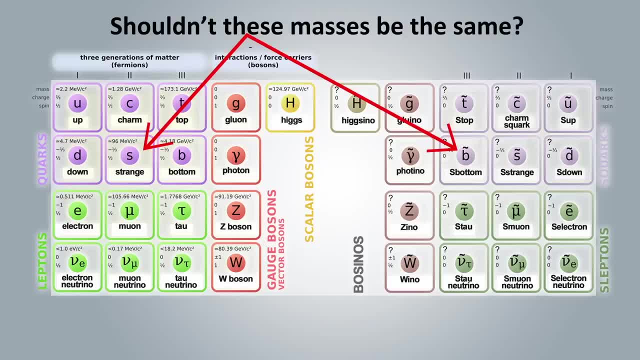 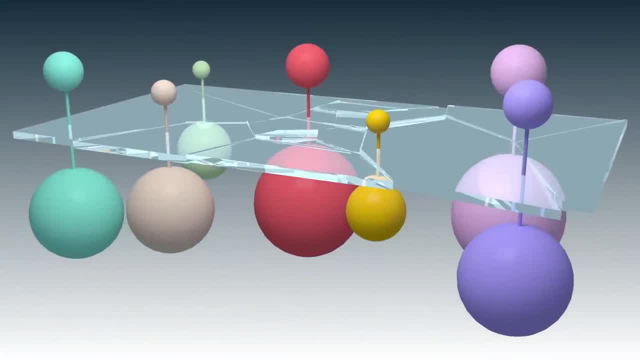 but just with some different spins corresponding to fermions and bosons. Well, in physics, symmetries exist, but they can also be broken. This, for example, is true for the electroweak force, The force particles involved in electromagnetism, and the weak 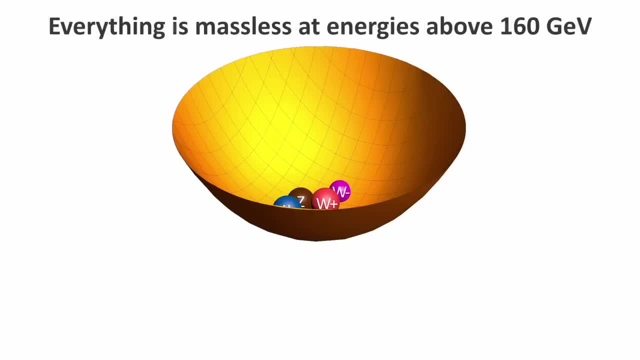 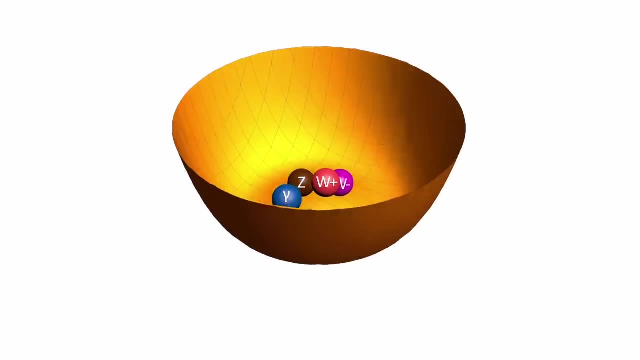 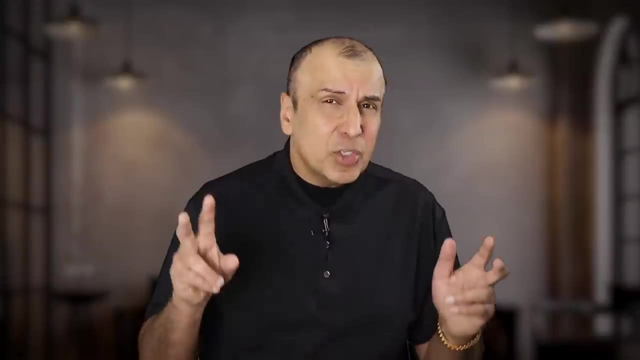 force are photons, W and Z bosons. They were theorized to all be massless, meaning their bare mass was zero. But the symmetry associated with those particles is broken by the Higgs field. That's why the Higgs field was theorized to exist. The idea is that superness could be. 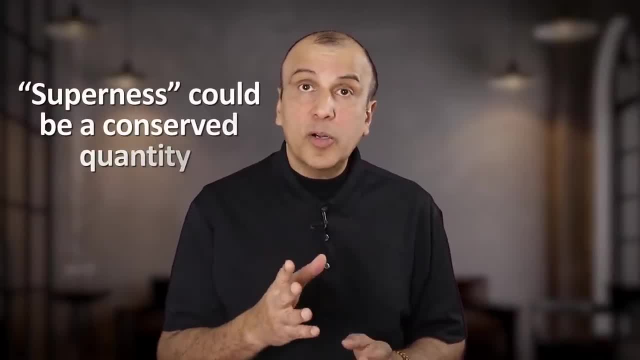 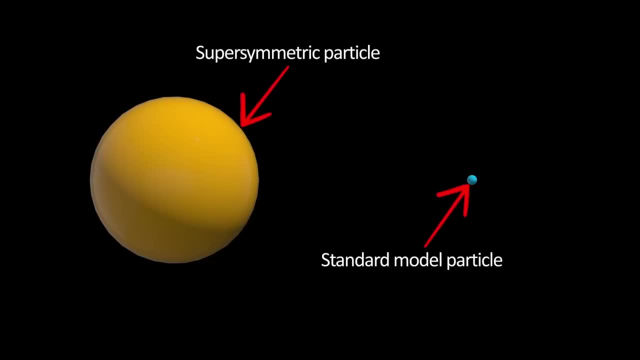 a conserved quantity like charge or energy. Superpartners would then not be able to decay to the ordinary fundamental particles of the standard model that we see, so they would be stable. So why haven't we handed out the Nobel prize for supersymmetry already? Well, because 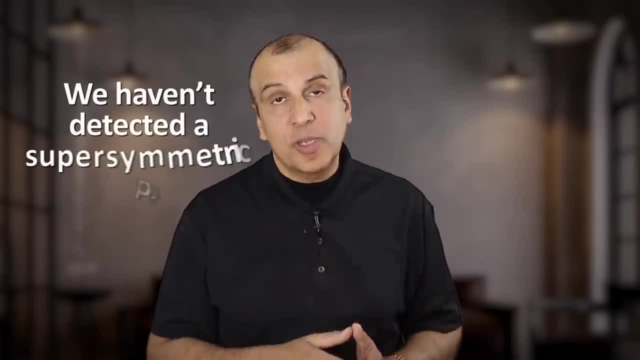 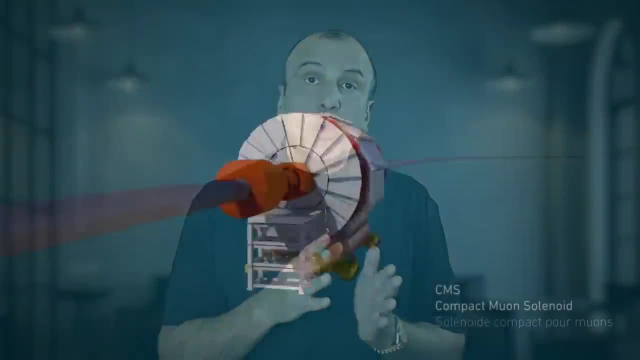 it's only a theory and we haven't discovered a single supersymmetric particle, But there could be two good reasons why we haven't detected them. The first reason, as I stated already, could be because the particles are simply so heavy that we can't produce them in our best accelerators, The 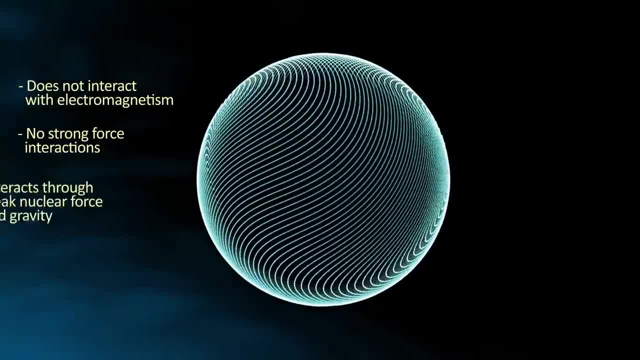 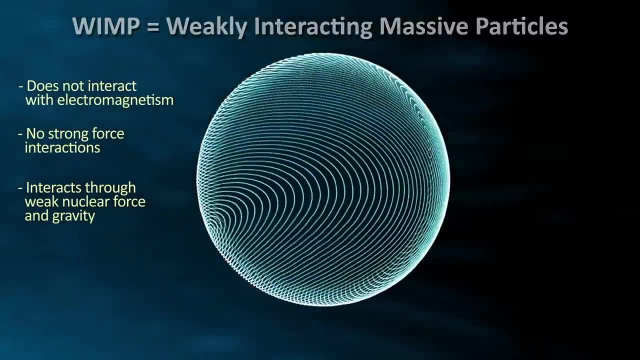 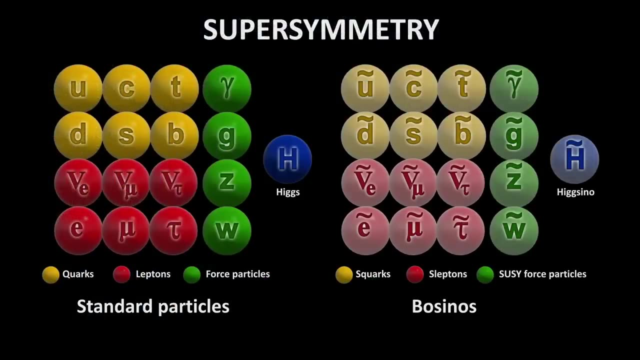 second reason is that if they are indeed dark matter particles, then they must be WIMPs or Weakly Interacting Massive Particles. So we could have produced these but simply not detected them because their interactions are so weak or rare. The math and concepts are quite clever, and the 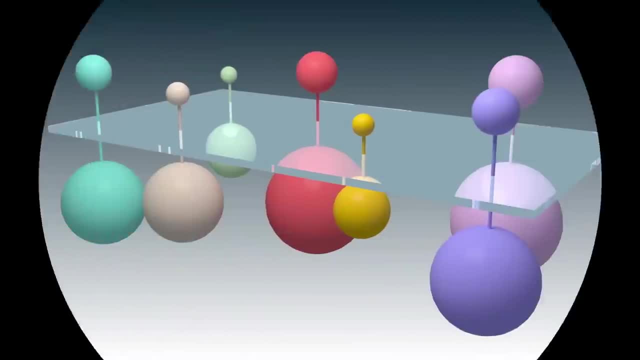 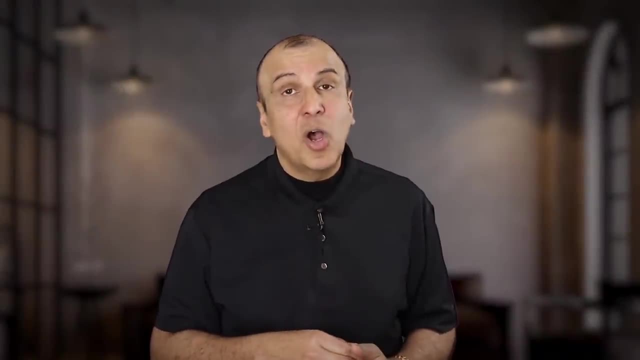 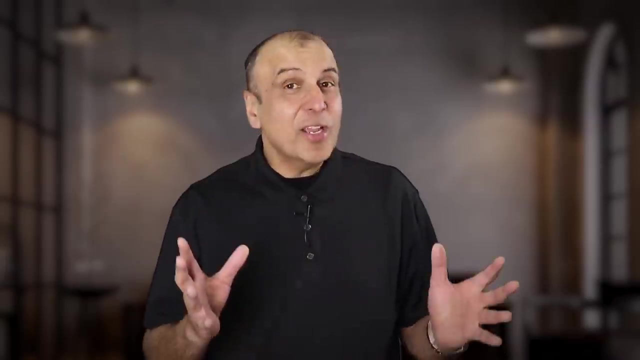 theory could explain some important aspects of physics. As time passes, though, it seems less and less likely to be correct, But all hope is not lost, because all we have to do is detect one of them, And that would bring us much closer to a theory of everything. A theory of everything, and. 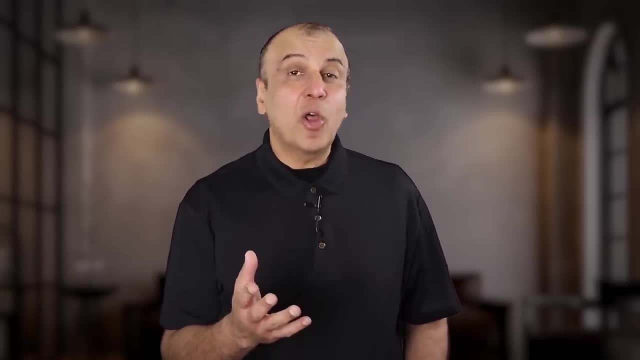 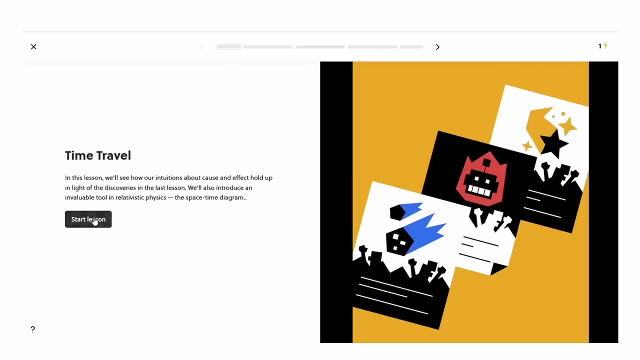 that's why supersymmetry is a very complex subject, So don't fret if you found yourself a little lost as I was explaining these ideas. What I've found is that an understanding of the fundamentals of science is crucial to understanding the most complex ideas. 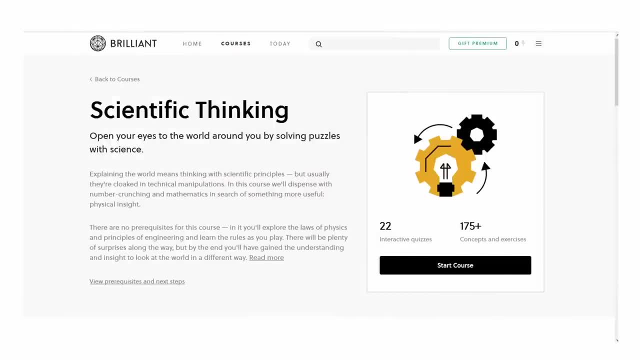 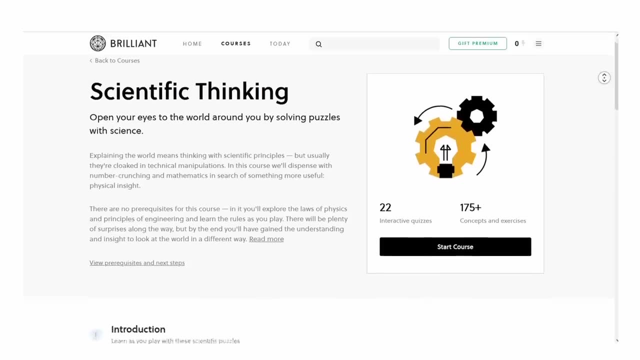 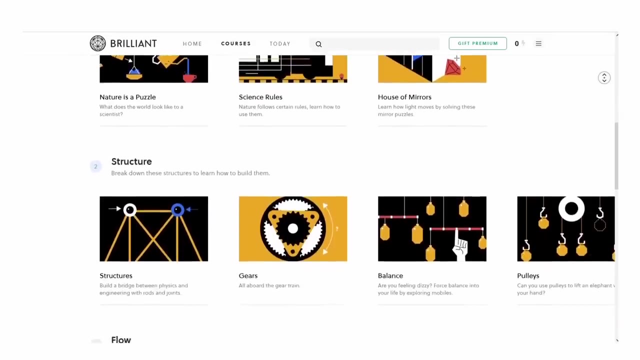 There's a course available on brilliantorg, today's sponsor, that I think can really help anyone better comprehend complex subjects like this called scientific thinking. I love this course because it goes through some of the basic fundamental ideas in science and this, I feel, is really helpful in building a basis for a better understanding of more complex 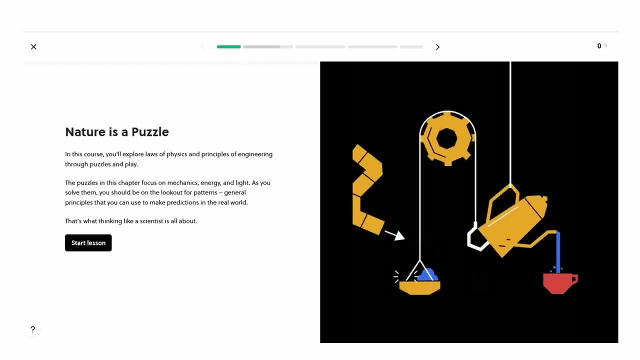 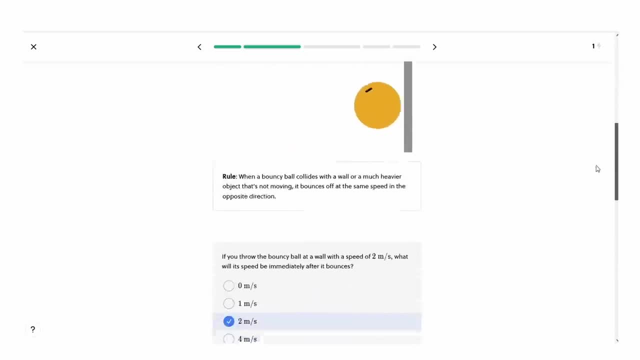 ideas. It's a 21-part course that explains how to think with scientific principles without focusing so much on the mathematics And, as always Brilliant, makes the learning process fun by inserting interactive quizzes after learning every new concept. This keeps you engaged and helps you. 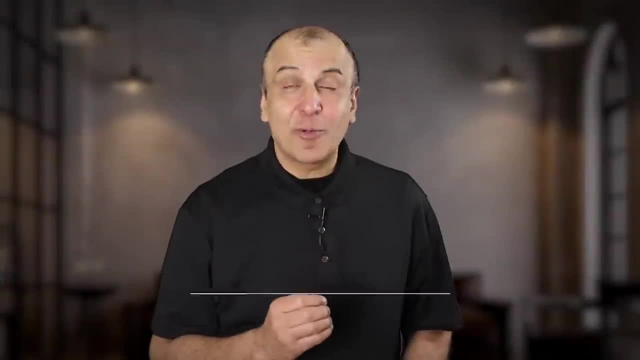 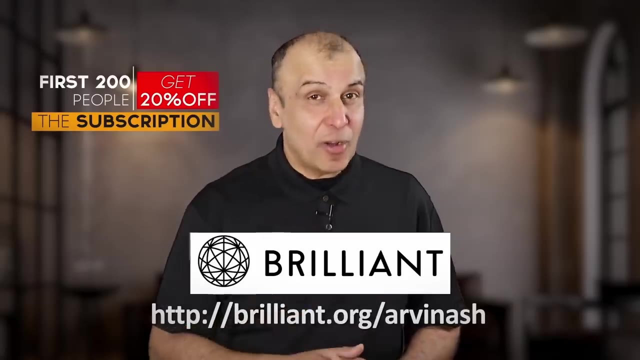 retain more information long term. Brilliant has a special offer for Arvin Ashbyers right now. Get started for free by clicking the link in the description. The first 200 people will even get 20% off your subscription. This is a great opportunity to give Brilliant a try. 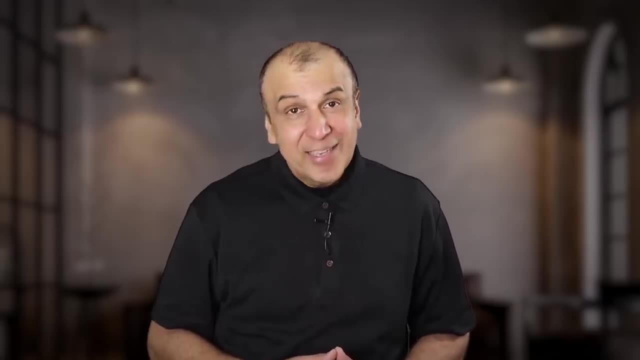 so be sure to click the link in the description And if you have any questions for me or any of our viewers, please leave them in the comment section. I try to answer all interesting questions. I'll see you in the next video, my friend. 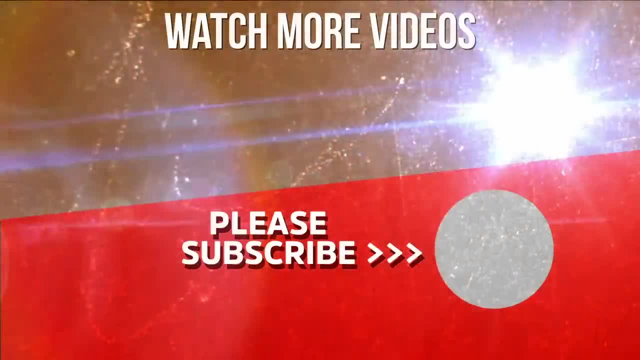 Thanks for watching and I'll see you in the next video, my friend.